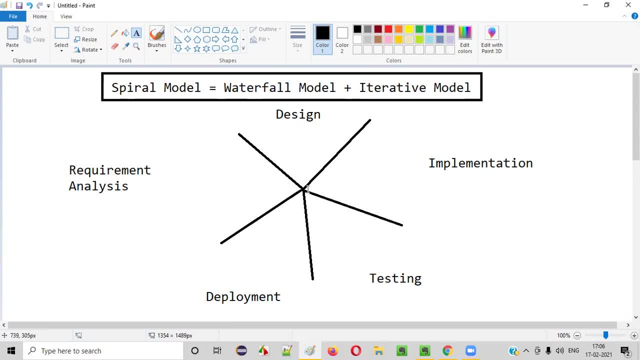 waterfall model Here. you see all the phases of waterfall model are there here. That means let's say, let's say there's a company like Microsoft, For example. guys, okay, let's say there's a company like Microsoft, They thought of developing a software. Say they want to develop this. 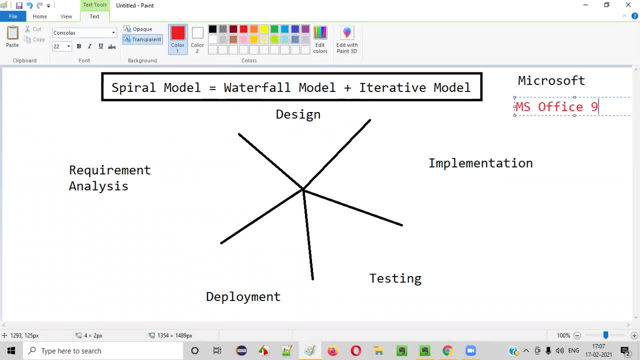 MS Office software for version 95. The first version of MS Office, let's say 95, they want to develop Later. they are going to try to, unless they don't have hardware, Okay. so you see, they are designing all the how this software is being. 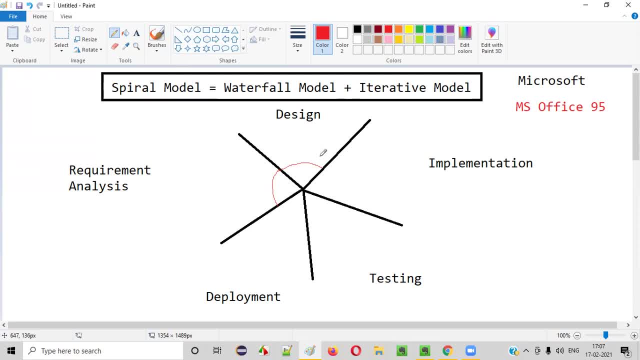 created all the requirements. Once the requirements analysis phase is completely completed, that is, all the requirements are fully gathered and fixed, then only they will move to the design phase. they will design all these requirements: low-level, higher-level designs. 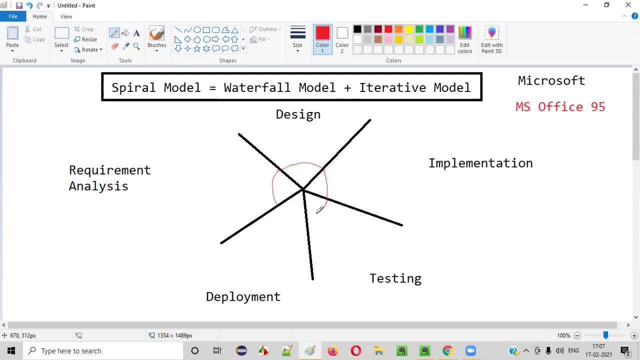 They will design for all these requirements. Once the design phase is roughly completed- cinco minutos hace, with animation- they will move to the testing phase. once this complete testing for this first set of requirements for this ms office 95 is completed, then they will move to the deployment phase. okay, they will deploy. 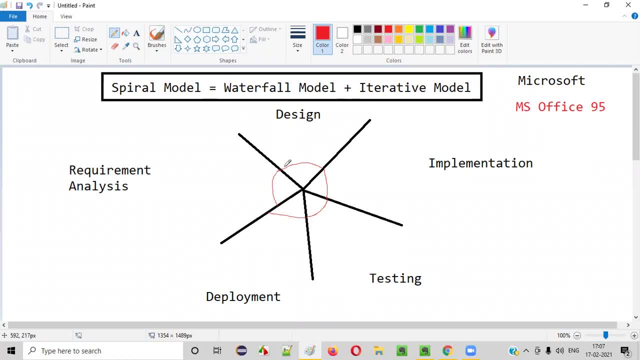 it. so this is the first iteration. whatever the orange color you are seeing, here is the first iteration. in the first iteration the waterfall model is there right. in this first iteration, starting from requirements, design, implementation, testing, deployment, there is nothing but the waterfall model. now, so fine. finally, microsoft has released their ms office version 95 after. 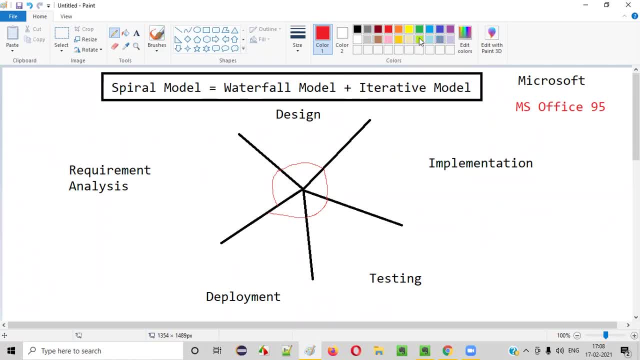 this deployment of this first iteration tomorrow. the same company, microsoft, thought of enhancing this existing software of ms office 95 and they want to release the latest version of microsoft ms office, that is, ms office 98. they want to release. okay, they want to develop and release. 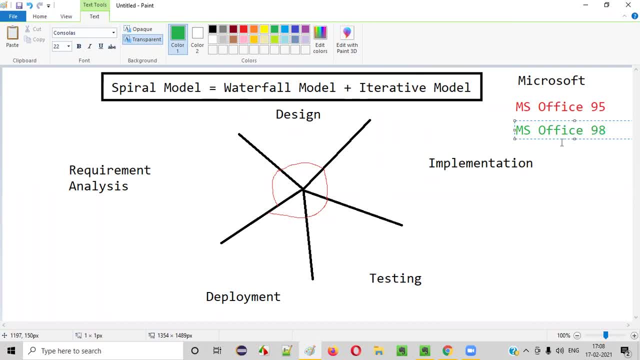 next version of software, ms office software, that is, ms office 98. for that again they will start with this, collecting all the requirements for this ms office 98, and then they will fully design all these requirements of ms office 98 98. then they will implement the 98, that is, develop the. 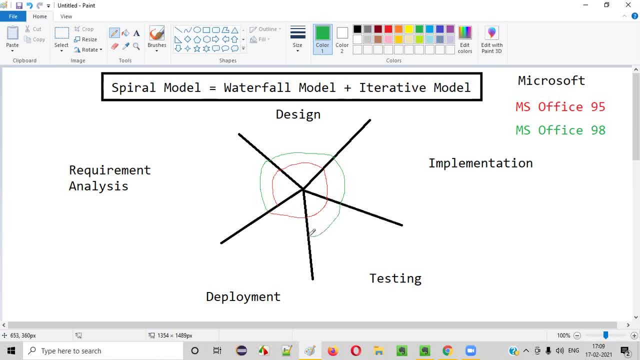 ms office 98. then they will fully test the ms office 98 software and they will finally release into the market, deploy and release into the market. so as part of the second iteration another waterfall model came here. there are several iterations in the first iteration. there is one. 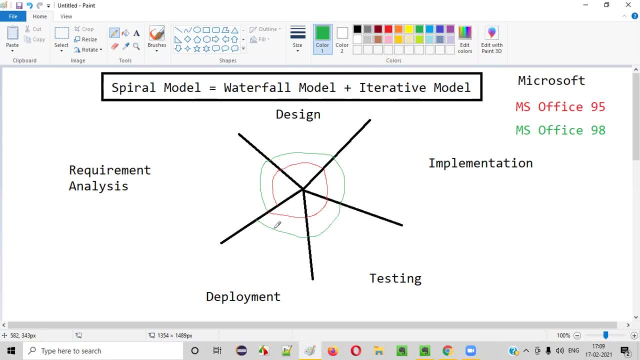 waterfall model. in the second iteration, which is represented in green color here, there is another waterfall model. right for every iteration there is a waterfall model, so which is together called a spiral model. guys, okay, waterfall iterative model, that is nothing but the spiral model. for every iteration there is a product or latest version getting released into the market. 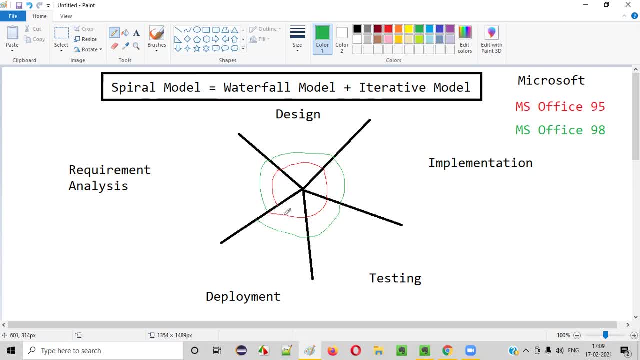 you. the first iteration, first version of the product got released. the second one in the second iteration, second version of the product got released. tomorrow the microsoft has decided to release another version of the software, another latest version of the software, let's say ms office 2000 they want to release. okay, 2000 they want to release. so again, it will start here, right. 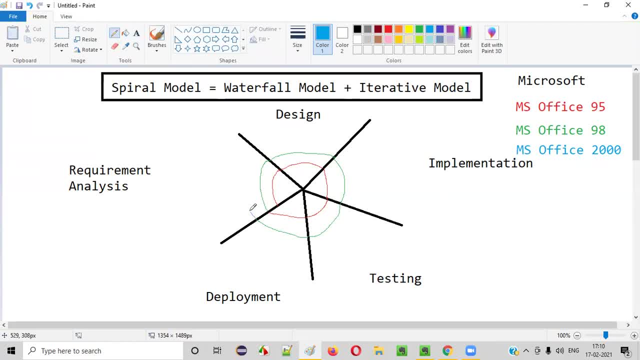 again. it will start here. they will gather all the requirements, then design it, then then develop it, then test it completely, then deploy it. The third iteration: also waterfall model is there again. In every iteration there is a waterfall model which is nothing but a spiral model. 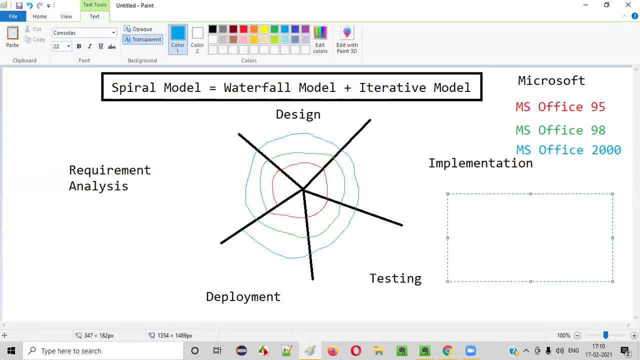 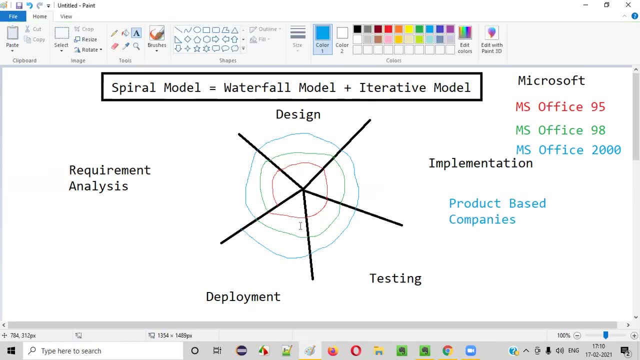 Generally, this kind of model is followed by the product-based companies. Product-based companies. they follow this model for releasing the several versions of the product, For releasing the several versions of the product. product-based companies like Microsoft will be following this kind of spiral model guys. 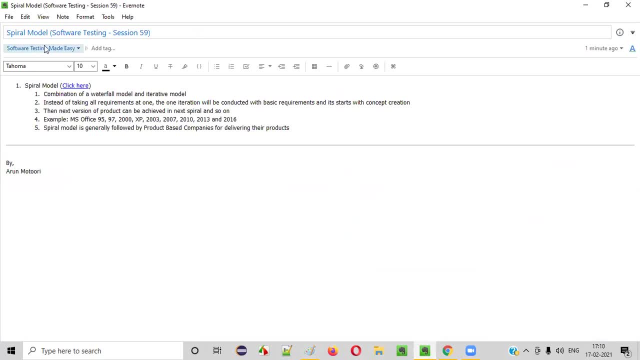 So hope, guys, you understood what exactly is this spiral model. Spiral model is a combination of the waterfall model and iterative model. Generally, the product-based companies deliver their products version by version, latest versions by using this spiral model. So that's it for this session, guys. Thank you Bye.